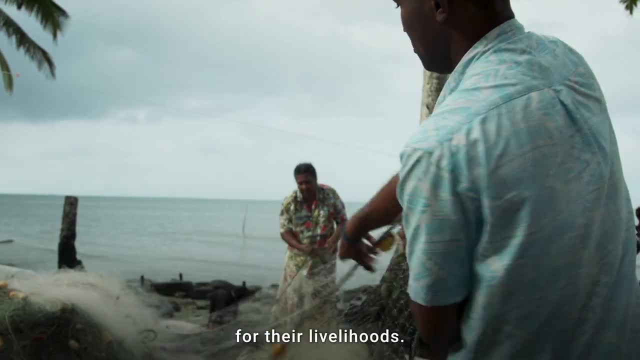 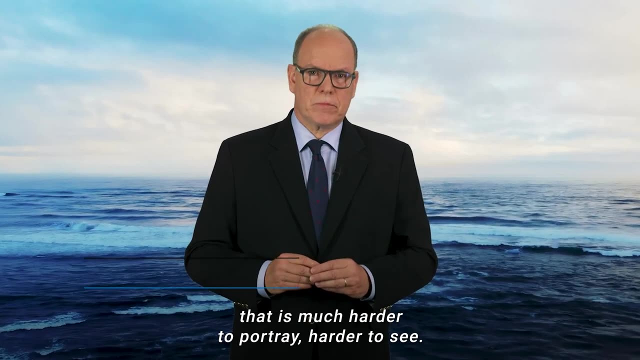 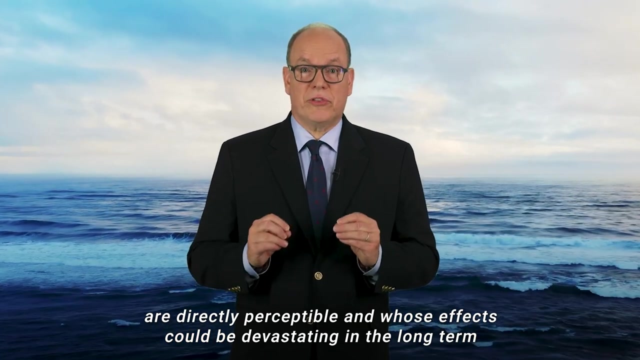 Over 3 billion people depend on the ocean for their livelihoods. Ocean acidification is, of course, a phenomenon that is much harder to portray, harder to see, Yet it is now a reality whose economic consequences are directly perceptible and whose effects could be devastating in the long term for many sectors. 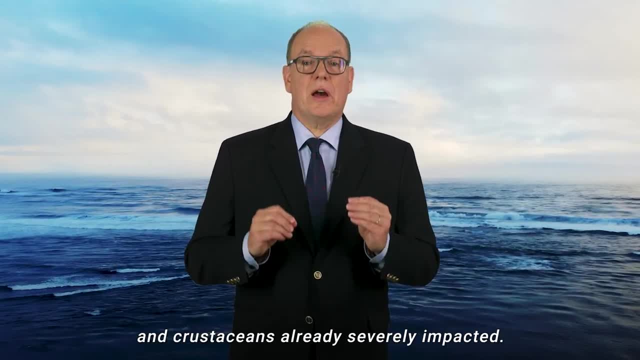 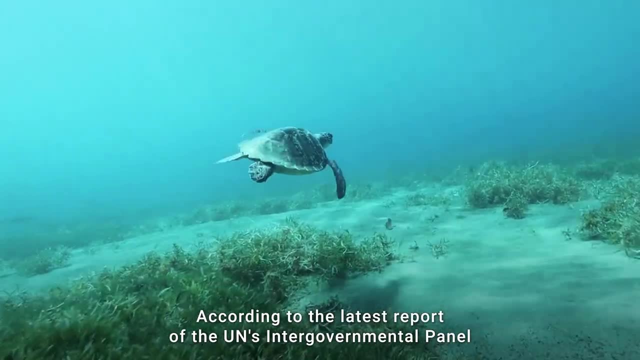 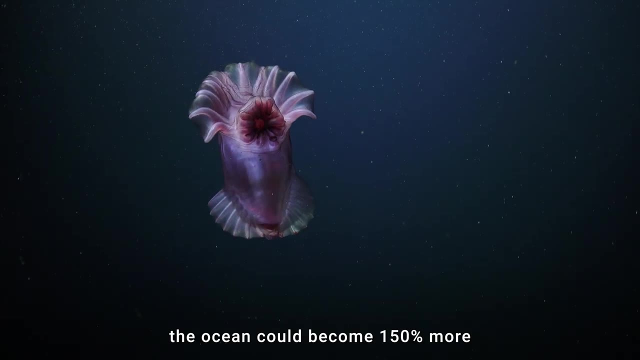 starting with farming and harvesting, But it is also the impact of many shellfish and crustaceans already severely impacted. According to the latest report of the UN's Intergovernmental Panel on Climate Change, scientists predict that by 2100, the ocean could become 150% more acidic. 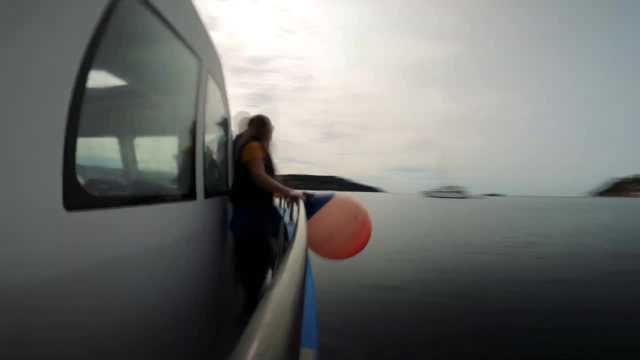 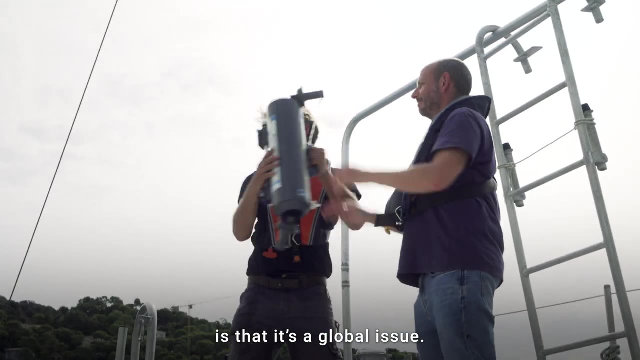 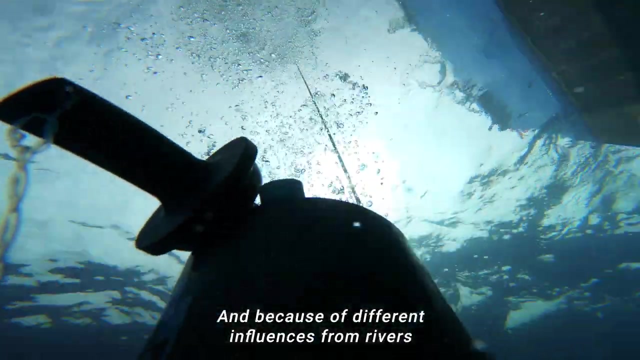 and affect half of all marine life. There are many challenges to addressing ocean acidification, and one of the big ones is that it's a global issue. Oceans are completely all over the planet and, because of different influences from rivers and the ocean chemistry varies a lot regionally that if you measure ocean acidification in one 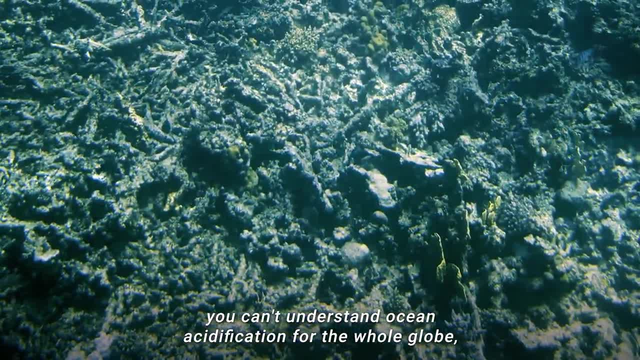 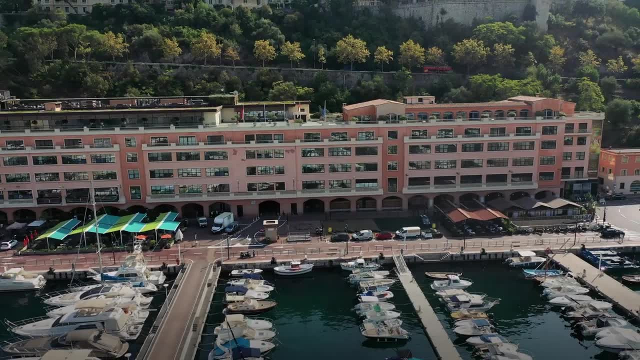 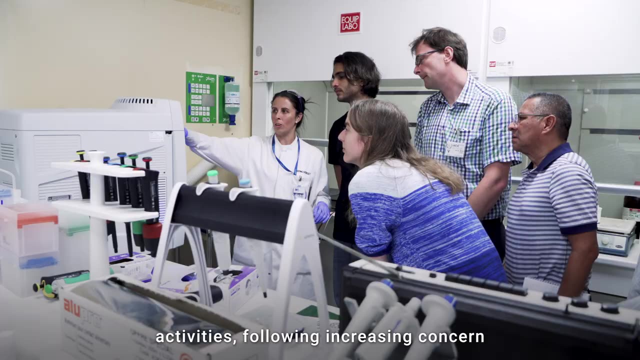 place, you can't understand ocean acidification for the whole globe, Which is why it's really important to have a global monitoring presence throughout the world for ocean acidification. This is why the IAEA runs a center to drive global ocean acidification activities following. 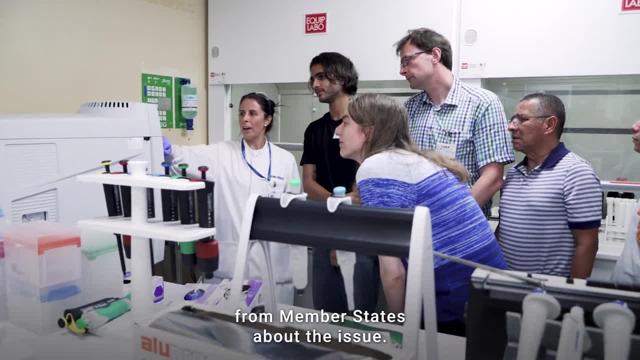 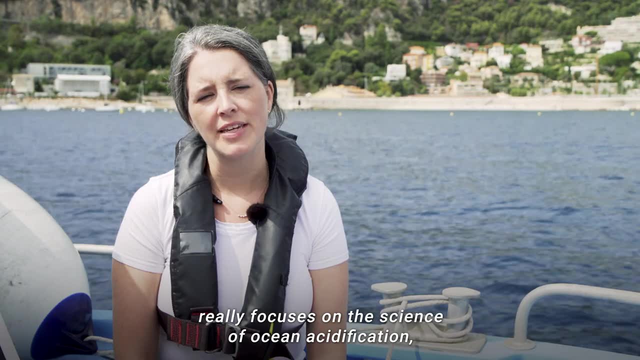 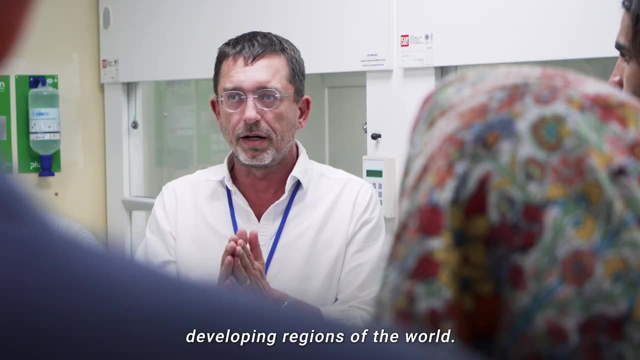 increasing concern from member states about the issue. At IAEA, the Ocean Acidification International Coordination Center really focuses on the science of ocean acidification, as well as communicating the dangers of this issue and building capacity in really vulnerable developing regions of the world. 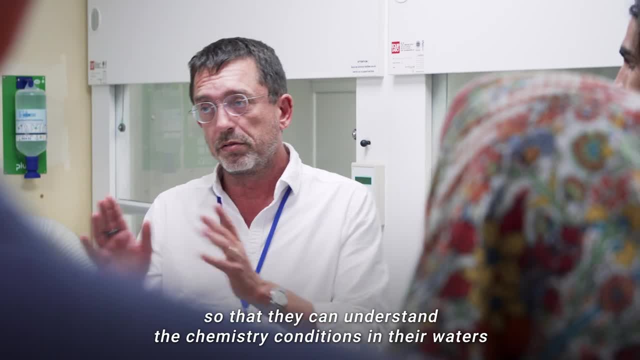 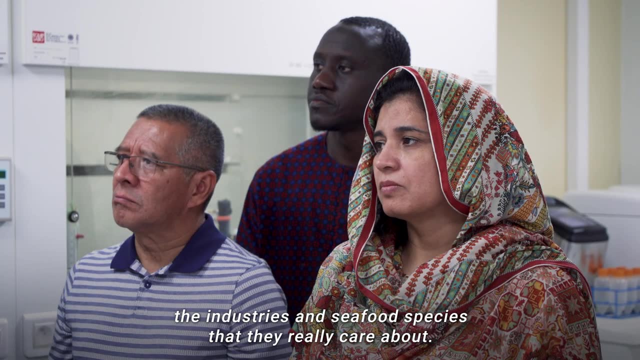 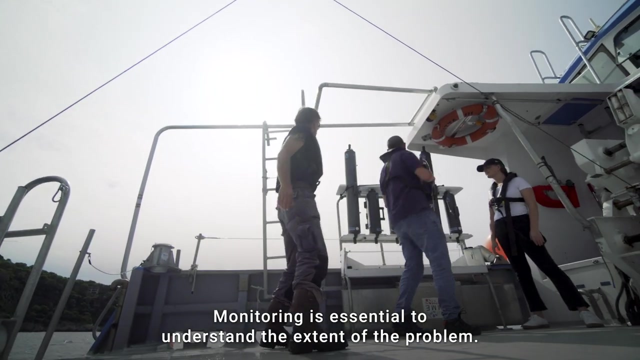 And this is really crucial- so that they can understand the chemistry conditions in their waters and then make projections about how this chemistry is changing and how it will impact the industries and seafood species that they really care about. Monitoring is essential to understand the extent of the problem, But is there anything that can be done concretely to combat ocean acidification? 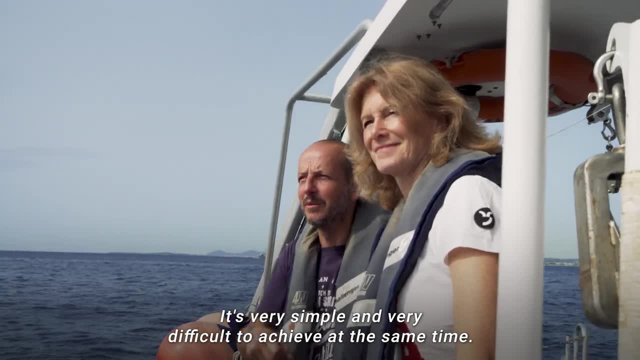 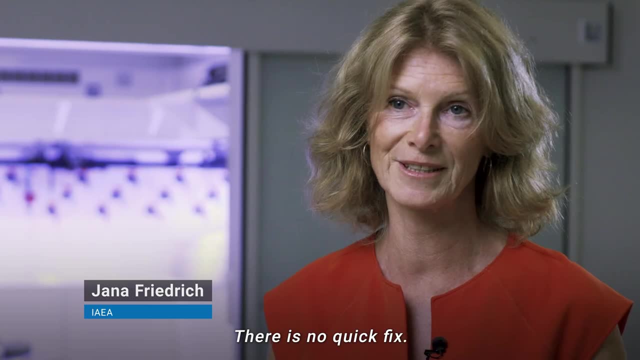 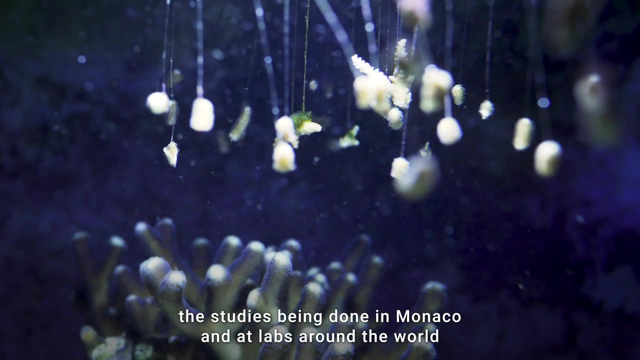 It's very simple and very difficult to achieve at the same time. The simple solution is: avoid emissions and decrease energy consumption. There is no quick fix Alongside global momentum towards the need to reduce carbon emissions, the studies being done in Monaco and at labs around the world.